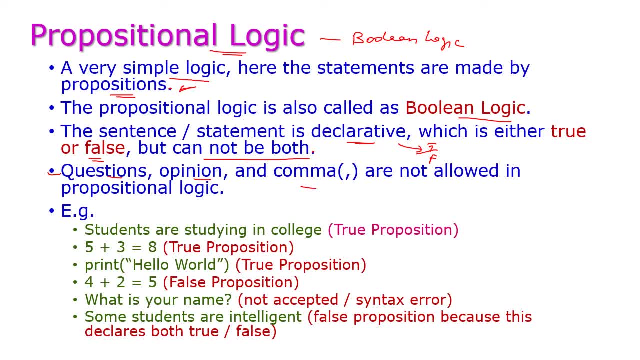 The questions, opinions and commas are not allowed in the statements or sentence here. We should not allow any questions, opinions or commas in the statements. We will see some example sentences for this propositional logic. The first one is: students are studying in the college. 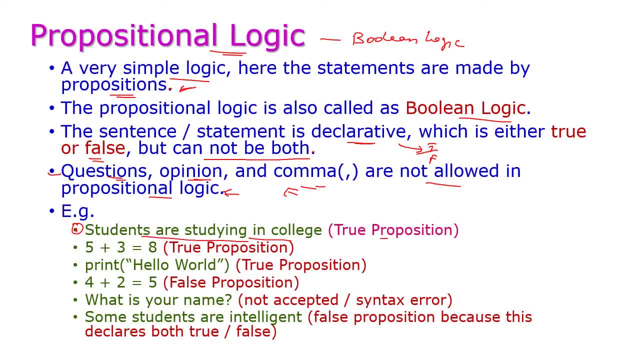 Students are studying in the college. So this is true proposition. All the students will study only in the college. Next, 5 plus 3 is equal to 8. So this is a mathematical sentence. So this is true proposition. 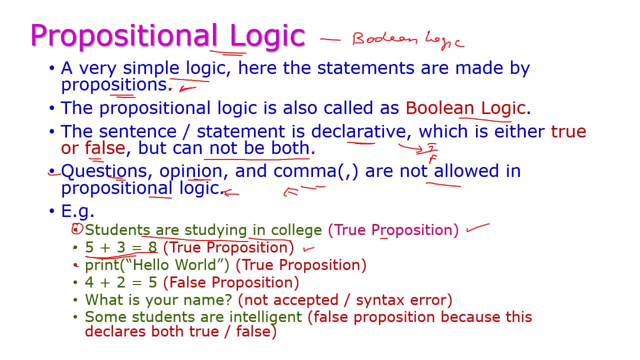 And next one is print of hello world. Print of hello world. This is one of the programming language syntax, For example Python, So this is also acceptable statement, True proposition. And the next one: 4 plus 2 is equal to 5.. 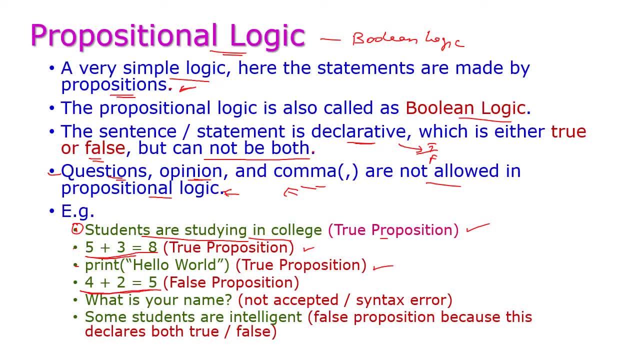 So this is true proposition. So this is a mathematical statement, but the result is false. So this is false proposition. And here, what is your name? What is the questionary word, Isn't it? So we should not allow this. what in the propositional logic? 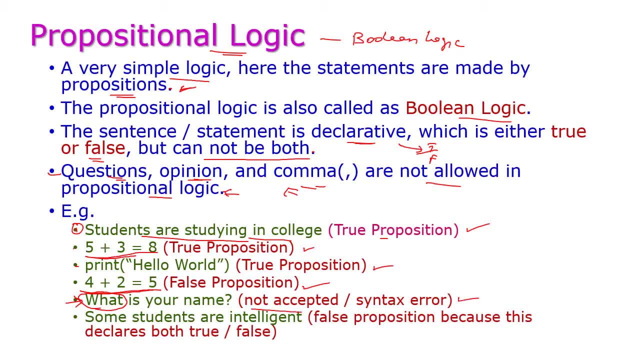 So this is not accepted. We will get the syntax error. And next, some student are intelligent, Some student are intelligent. So in this statement, some students are intelligent is true. And also, what about the other students? The other students are not intelligent. 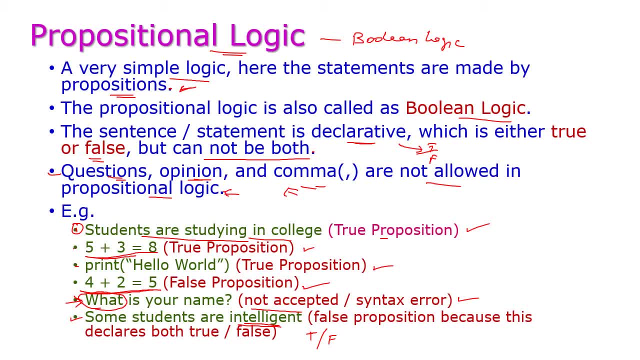 So false, False proposition, because this declares both true and false. Okay, this particular statement will accept both true and false. And also we cannot accept this particular statement in the propositional logic. So syntax error. Syntax error will come here. 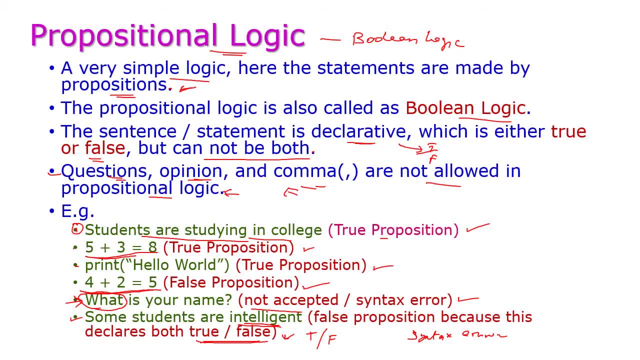 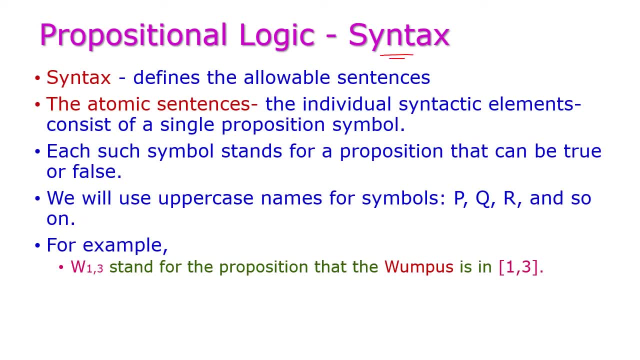 Okay, so these are the definition of propositional logic, And next we will see the syntax for this propositional logic. What is meant by syntax? Syntax defines the allowable sentences. Okay, that will define the grammar of particular logic. So the sentence should be accepted by this grammar of logic. 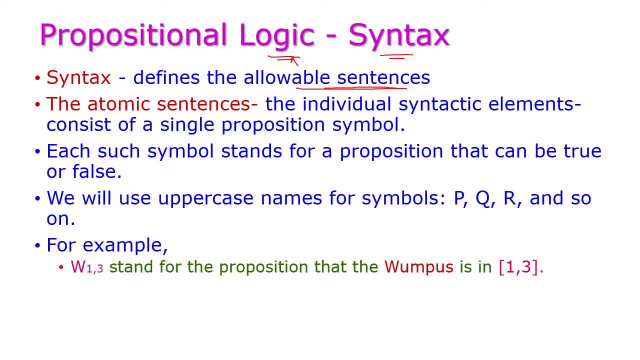 Then only the sentence will be accepted. Okay, so this is called as syntax. Syntax defines the rule for constructing a sentence, And here we are having two types of sentences. First one is atomic sentence- Atomic sentence And second one is complex sentence. 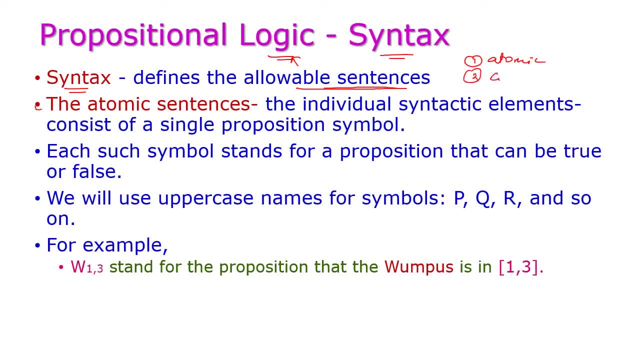 Complex sentences. First, let us see the atomic sentences. Okay, The individual syntactic elements consist of complex sentences. Okay, The individual syntactic elements consist of complex sentences. Okay, The individual syntactic elements consist of single propositional symbols. This is called as atomic sentence. 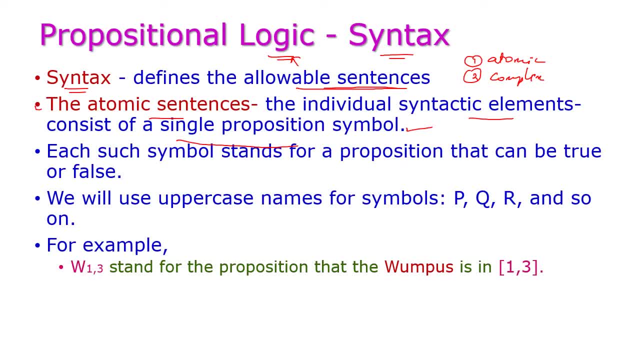 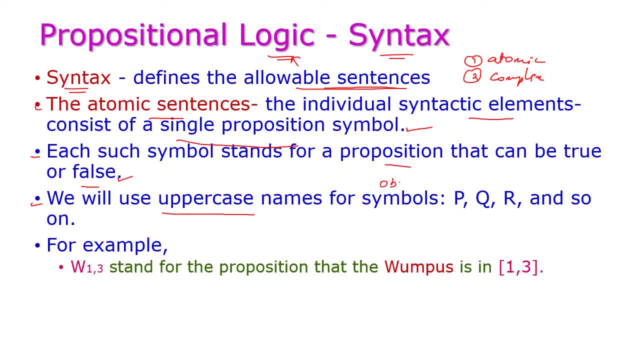 The symbol represents some objects. Okay, So the symbol represents some objects represent some objects. so p, q, r and so on. are the symbols right here? example w of 1 comma 3. w of 1 comma 3: here w is a symbol. 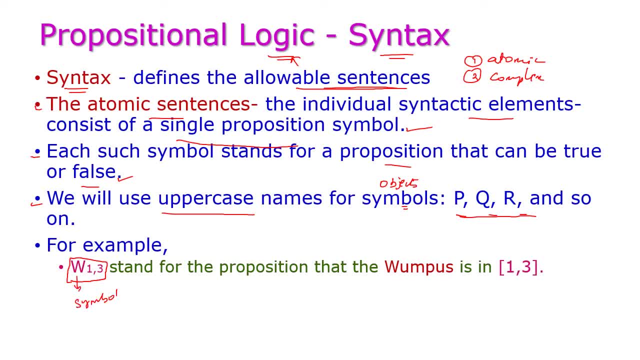 okay, which stands for the proposition that wampus is in the position 1 comma 3 in our wampus world example. wampus may be in 1 comma 3, for example. here wampus is here, so that is what wampus of 1 comma 3, so this is an acceptable statement in the propositional logic. 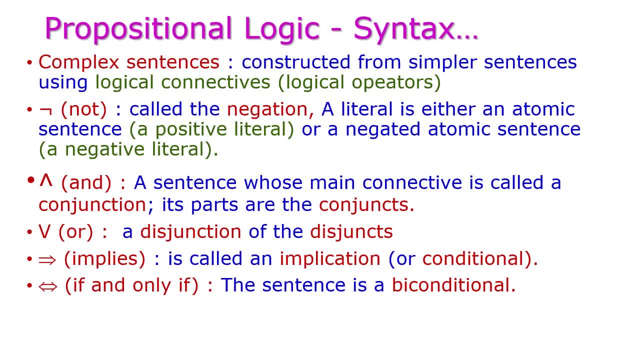 the next type of sentence is complex sentence. okay, the complex sentences constructed from the simpler sentences. the next type of sentence is complex sentence. okay, the complex sentences constructed from one or- sorry, two or more simpler sentences by using logical connectives, or otherwise called as logical operators. okay, so here we are having five logical operators. 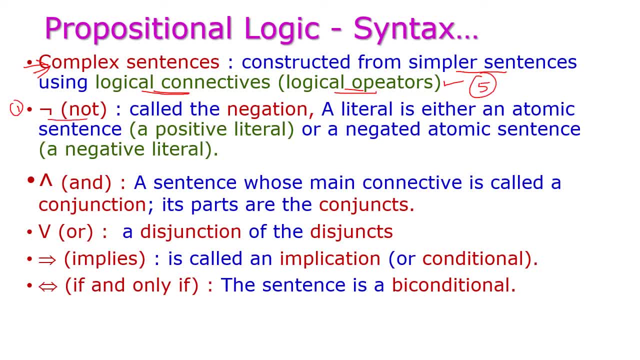 the first one is not okay. the symbol is this one: okay. this is called as negation. a literal is either an atomic sentence- that is, a positive literal or negated atomic sentence, or a negative literal. and the second one is, and this is the and operator right, the and sentence. 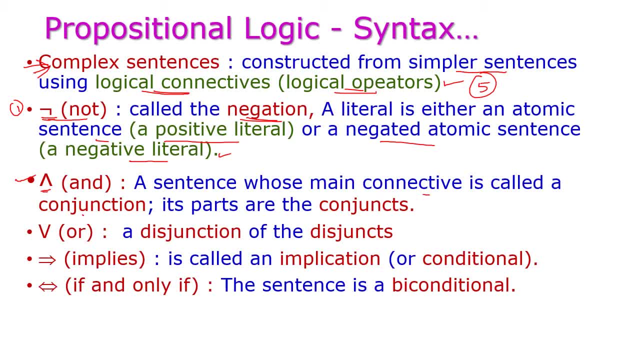 whose main connective is called as conjunction, so that this is the end- is called as conjunction here and its parts are conjunct. its parts are conjuncts a and b. okay, a and b are symbols, and here these symbols are called as conjuncts and this is the conjunction. 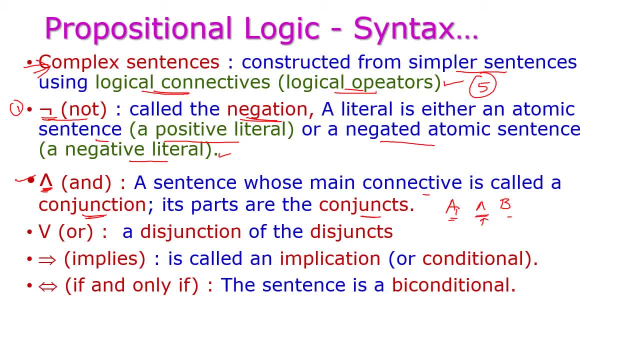 operator and the next one is r. the next one is r. so this is disjunction and the parts are disjuncts- a or b. either a is true or b is true, right, and the next one is implies, that is, the if, then operator, if, then operator or conditional operator. okay, this is implication. 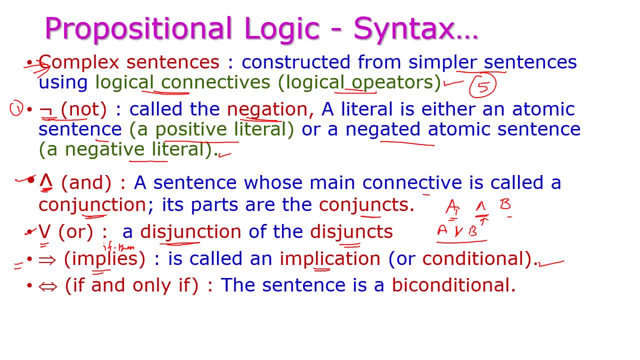 or conditional operator right. and the last one is biconditional if and only if, if and only if the sentence is a biconditional sentence, the operator is biconditional operator. so by using this logical connective we can connect the atomic sentences to make these complex sentences. 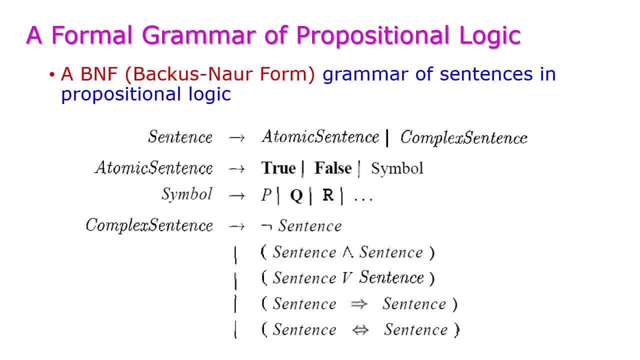 and next let us see the formal grammar of propositional logic. so here the grammar of propositional logic is bns, that is back a snore form, the grammar of sentence in the propositional logic. here it will accept the sentences. there are two types of sentences. first one is a sentence and the second one is a sentence. 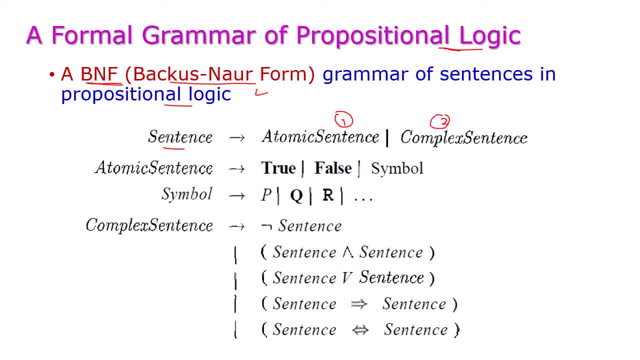 atomic and second one is complex sentences. atomic sentence consists of true, false or simply a symbol. okay, and here the symbols are capital letters, uppercase letters- okay, the uppercase letters represent the symbols and complex sentences. we can create the complex sentences by using logical connectives. by using logical connectives, we can connect the sentences. 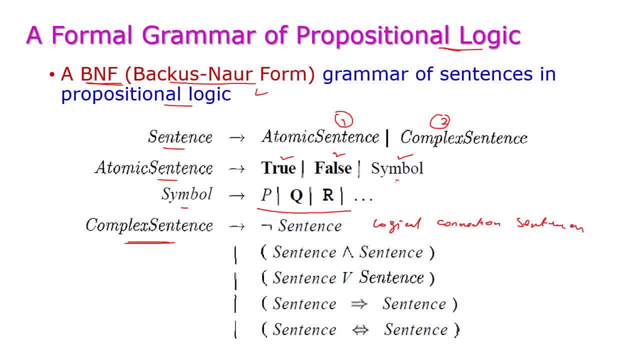 that is, atomic sentences. whatever sentence it may be okay, so what are the logical connectives we are having? first one is negation sentence or and conjunction. this is or that is disjunction, this is implication conditional statement and this is biconditional statement. okay, so by using 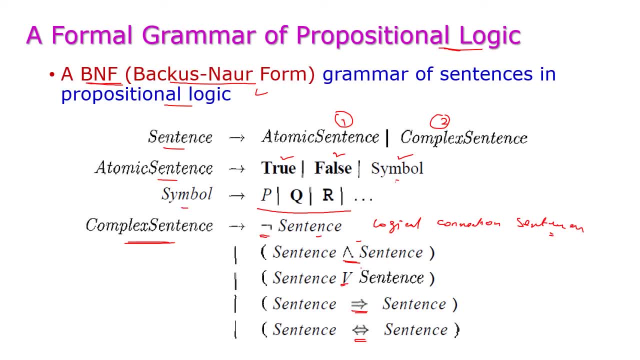 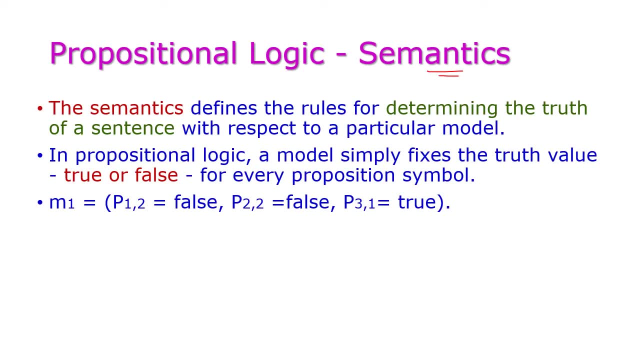 these logical connectives we can construct the complex sentences. And next we come to the semantics of propositional logic. Here the semantics defines the rules for determining the truth of a particular sentence, That is, with respect to a particular model. Here model is our problem. 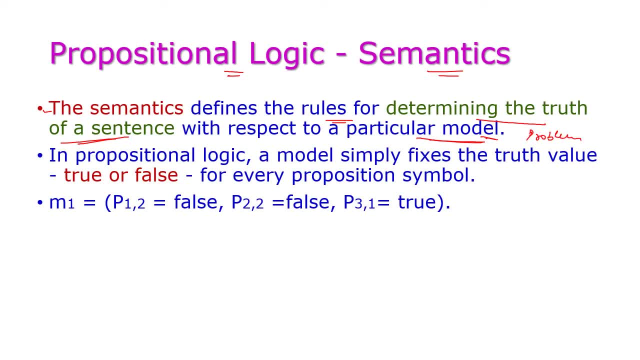 Model is our problem, or agent world, whatever it may be. In propositional logic, a model simply fixes the truth value. It may be either true or false for every propositional symbol. This is important. All the statements in that model should give the truth value. For example: 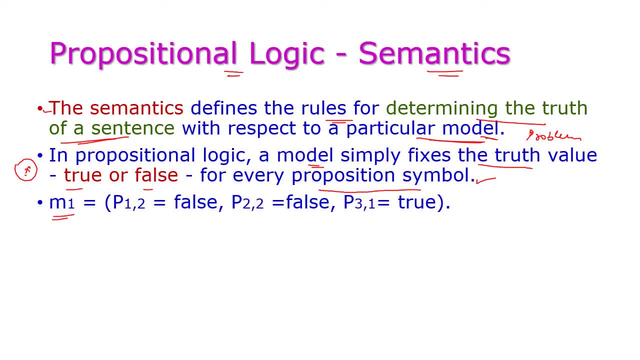 this is our model. In this model, p of 1,2, that is, pit is in 1,2, is false And pit is in 2,2 is false And pit is in 3,1 is true. So these are the statements that are available in this model. 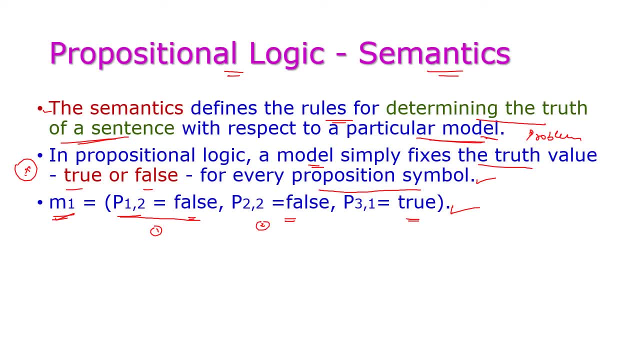 So this is first statement, Second statement And third statement. In all these statements, everything will give the truth value, Everything will give truth value. What are the truth value? we are having True, false, false. So in our statement, 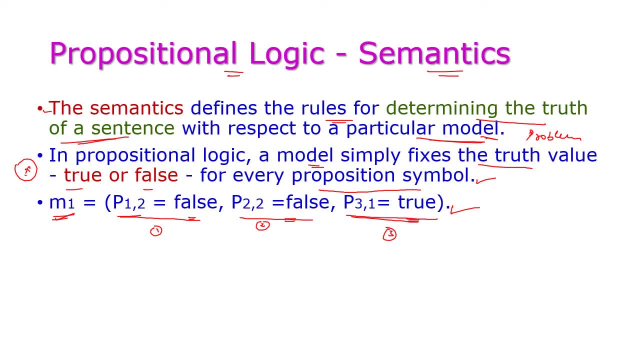 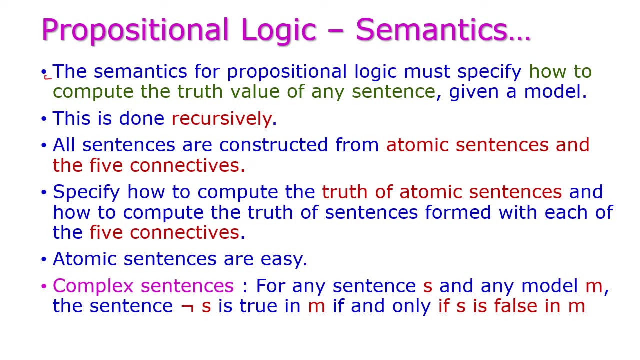 we can guess that pit is in 3,1.. But all these statements will be accepted by our model M1. Because all the models will give the truth value. And here the semantics for propositional logic must specify how to compute the truth value of any sentence. 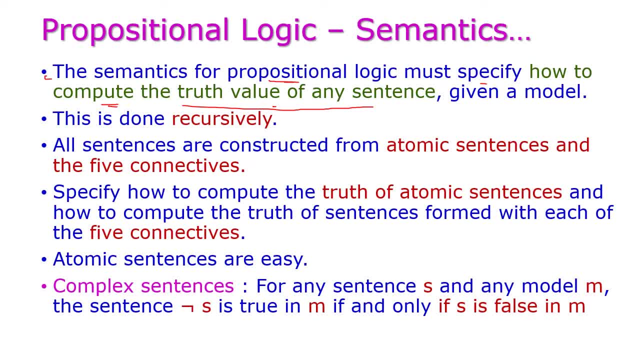 So we have to specify the computation of truth value of particular sentence which are given by a model, And at a single step we cannot get the truth value But recursively. if we do, then we can get the truth value. All the sentences are given by a model, So we can get the truth value. 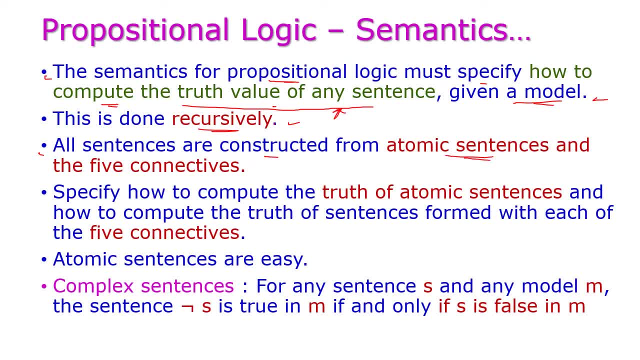 All the sentences are constructed from atomic sentences and the 5 connectives, Any one of the connectives or combination of connectives, And specify how to compute the truth of atomic sentences and how to compute the truth of sentences formed with each of 5 connectives. 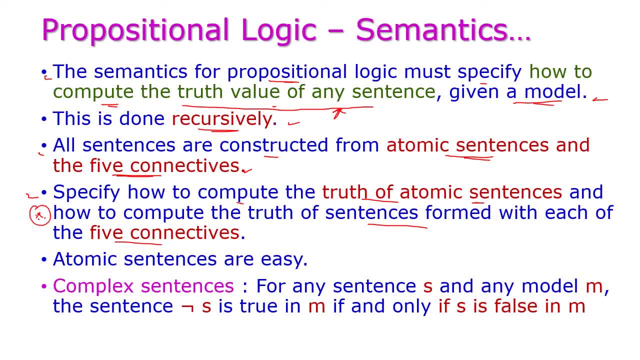 So we have to compute the atomic sentences, truth value. After that the combination of 5 connectives sentences. Also we need to compute, And here the truth computation of atomic sentences are very easy, But when come to complex sentences, 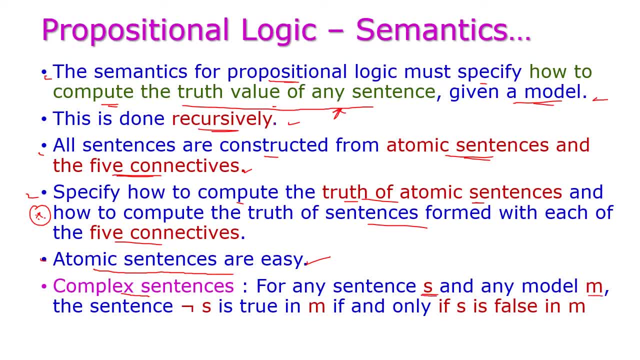 for any sentence S in any model M, the sentence not S is true. If the not S is true in our model M, if, and only if, S is false in model M- Okay, the truth value of S is false. Then only the not S is true. 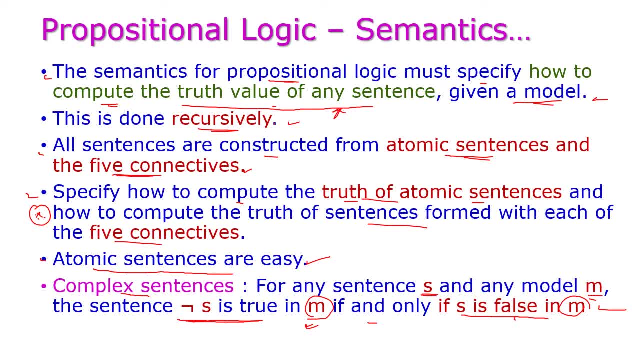 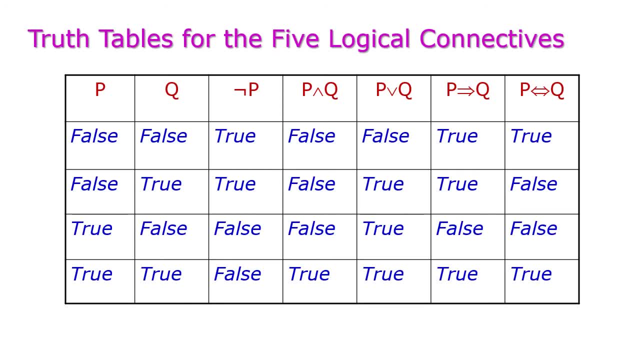 Likewise, we have to extract the information from the complex sentences. And here the truth table for 5 logical connectives. And there is nothing new in this table. Here we are having the object, P and Q. P and Q are symbols which represent an object. 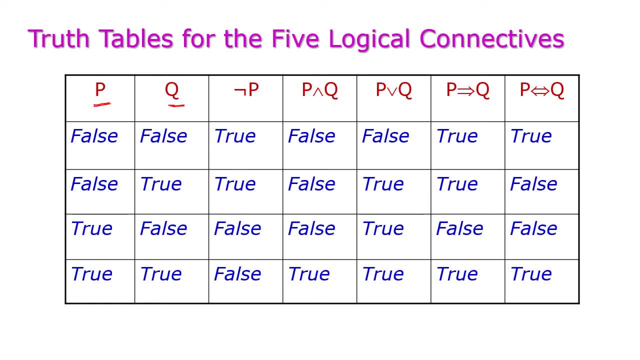 Here we are having the object: P and Q are symbols which represent an object, And here we are having all possible values of these two objects. Here we are having the object: P and Q are symbols which represent an object: True, False, False, False, False, True and True-True.